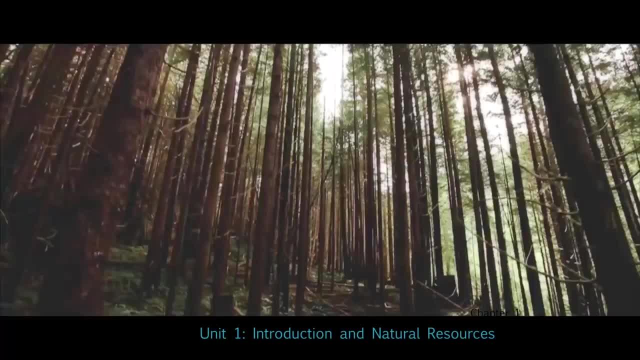 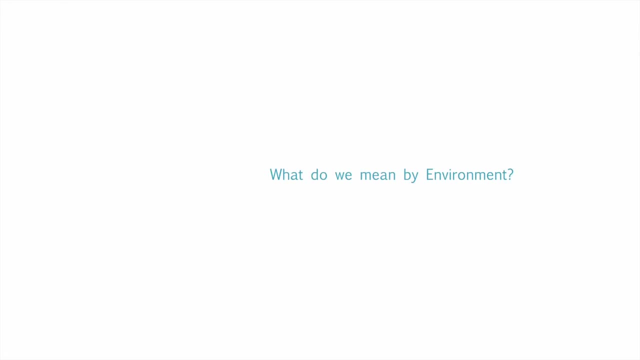 Unit 1: Introduction and Natural Resources. What do you mean by Environment? Environment is what surrounds us. There is a proper definition also: It is the sum total of all social, economical, biological, physical and chemical factors which constitute the surroundings of humans, who are both the creator and modulator of 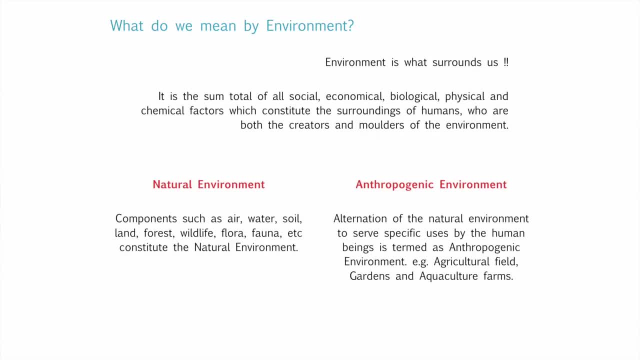 the environment. Environment is divided into two parts: natural environment and anthropogenic environment. Natural environment which exists naturally, like air, water, soil, land, forest, etc. And anthropogenic environment, which are manmade or alteration of the natural environment which serve a specific use by the human beings, For example agricultural fields, gardens. 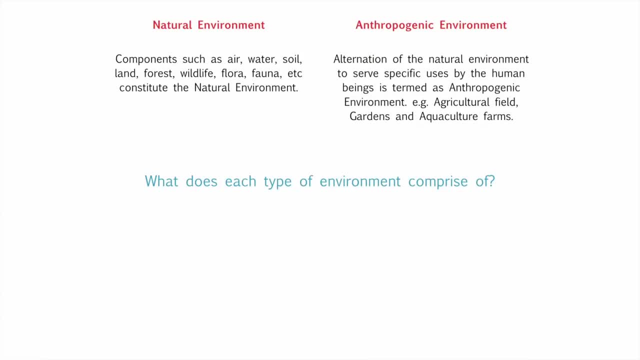 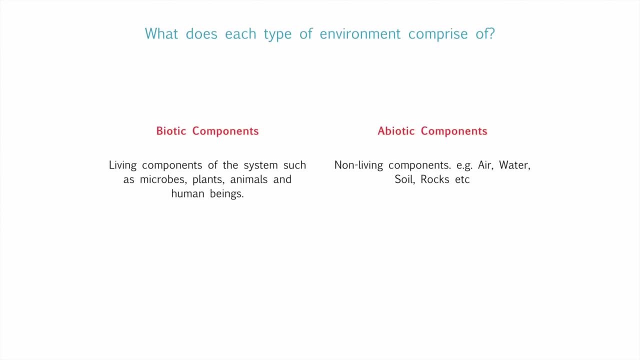 and aquaculture ponds, etc. Now, all these environments are consist of two basic components. They are biotic component and abiotic component. Biotic components are the living components of such a system, like microbes, plants, animals, etc. Abiotic components are non-living components, like air, water, soil, rocks, etc. 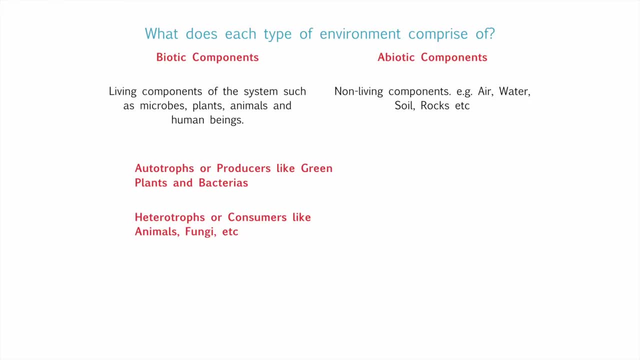 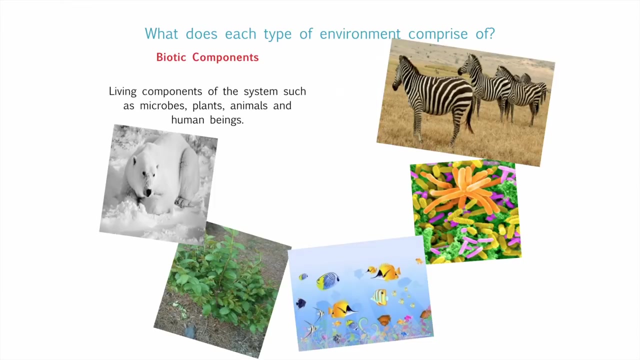 Biotic components are again divided into two parts: Autotropers, which are producers: They produce their own food, like grain plants and bacteria. Heterotropers, they are consumers and they depend on autotropers. component of the environment, like animals, punggys, etc. 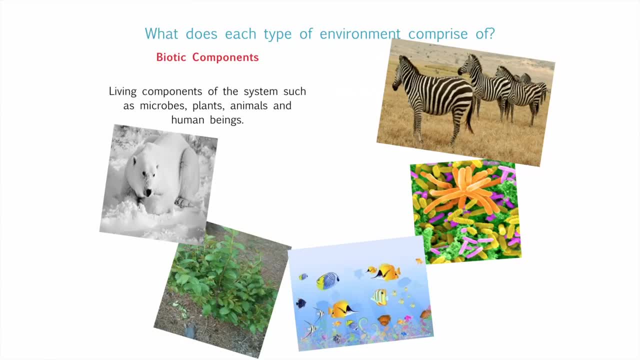 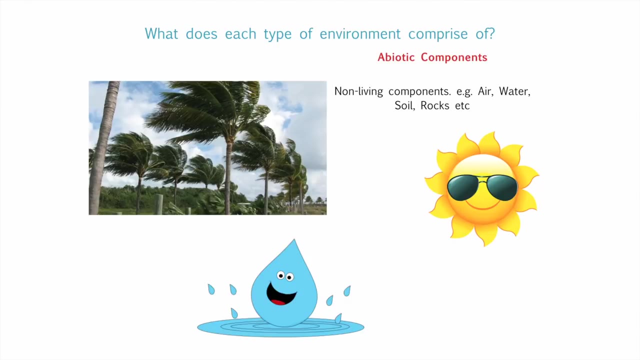 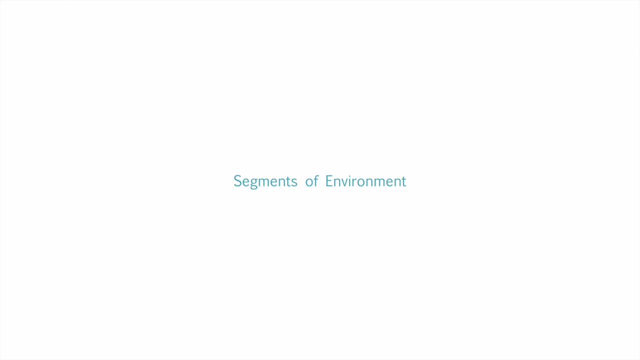 These are the examples of biotic components like animals, plants, sea creatures, microorganisms, trees and many more. These are examples of abiotic components like air, water, soil, etc. Now, what are the segments of environment? Environment is a very big thing and it is divided into different segments just to study. 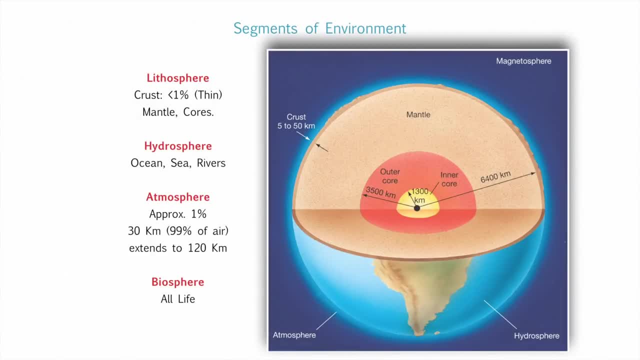 the environment. So main components are. main segments are Lithosphere, Hydrosphere, Atmosphere and Biosphere. Lithosphere is related to all the solid materials, which includes crust, mantle, core and all other solid materials available on the earth. hydrosphere is related to the water: water. 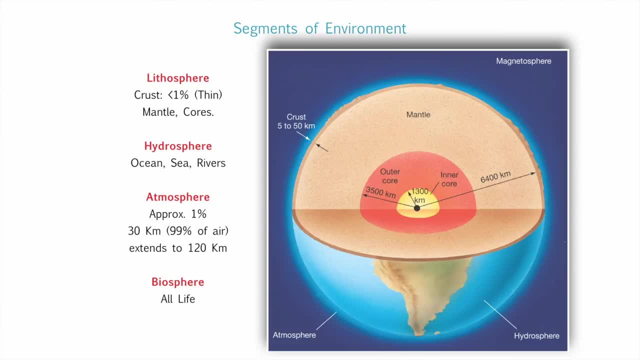 that means all the things related to ocean, sea, river will be included in hydrosphere and atmosphere is related to the gaseous state, so it extends up to 120 kilometer from the surface of the earth and it consists of all the gases. and finally, biosphere, which, which is the segment of 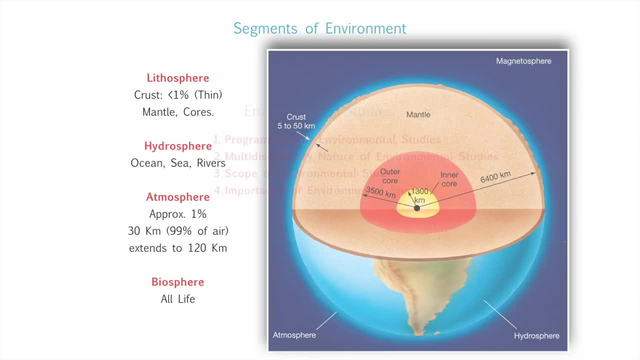 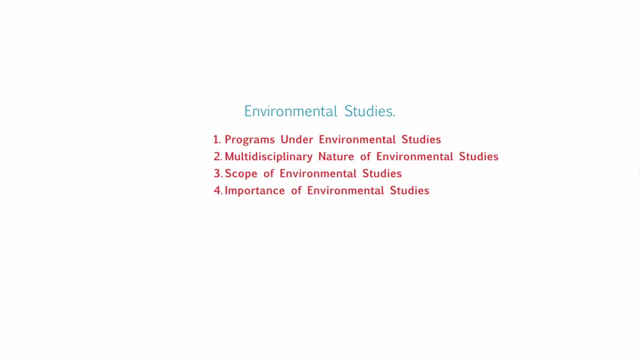 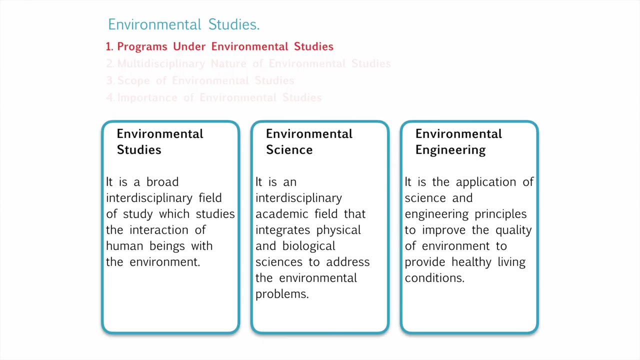 all living organisms, including all the lives. now environmental studies are divided into four parts where we are going to study the programs under environmental studies. it's multidisciplinary nature, scope of environmental sciences and importance of environmental studies. so first of all, programs. there are three main major program programs like environmental studies, environmental science. 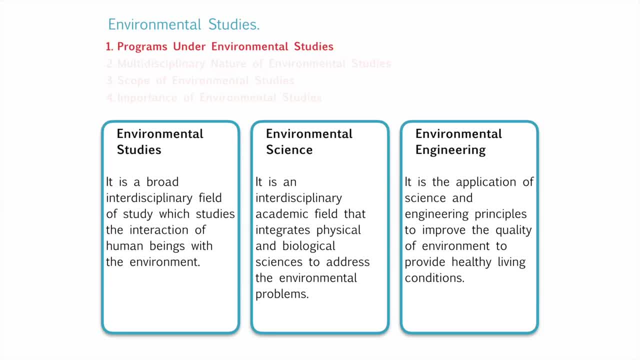 and environmental engineering. environmental study is the broad, interdisciplinary field of studying which studies the interaction of human being with his environment. it's the interaction of human being with the environment. secondly, environmental science. it is the science behind each and every environmental process. the basis of environmental interaction is Erm难. 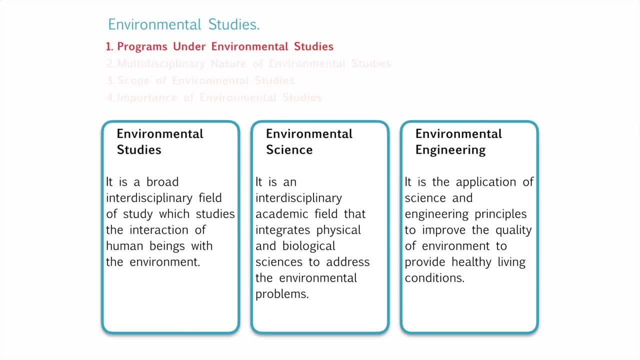 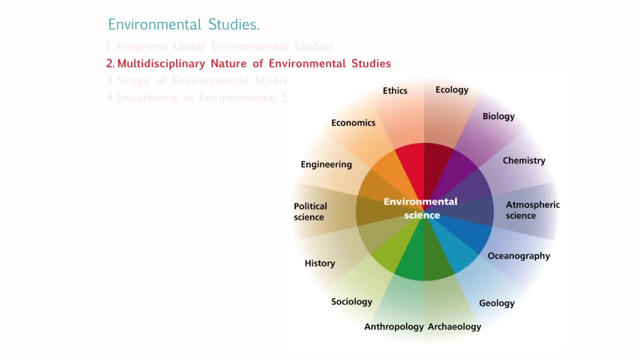 the basic science behind the environmental process. this can be physical, chemical or biological sciences, Physical, Chemical or atleast. and environmental engineering is related to the applied part of the environment, where we will study the science and engineering principles to improve Abang quality of environment and healthy living conditions. now, multidisciplinary nature, the environmental science as an environment with various environmental factors, the one that actively heal our environment. so i would like to summarize this into the diversity of of environmental science. what is environmental science and environmental society? login. 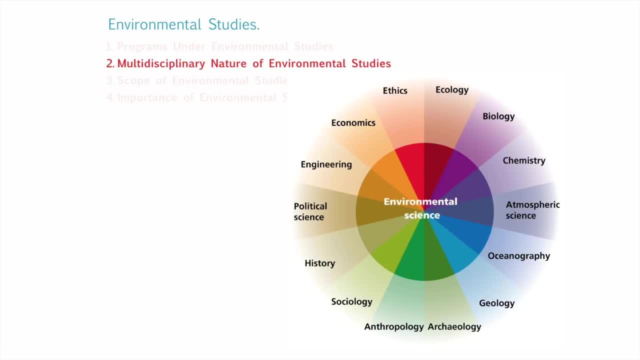 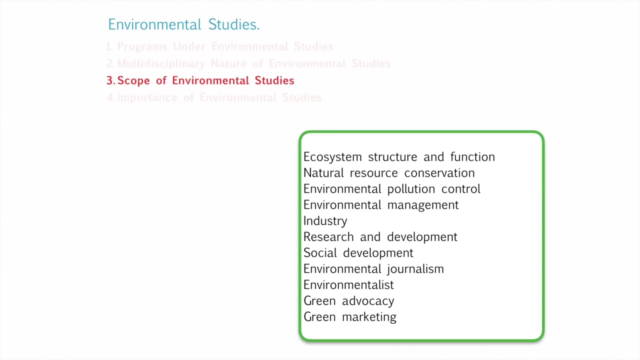 the environmental science consists of a lot, a very big field of environment which can be related to any other branch of the science- engineering or engineering. that's why it is multidisciplinary subject and we need to study all the things now. scope of environmental studies. when you study environmental studies, when we are taking a course of environmental studies, then 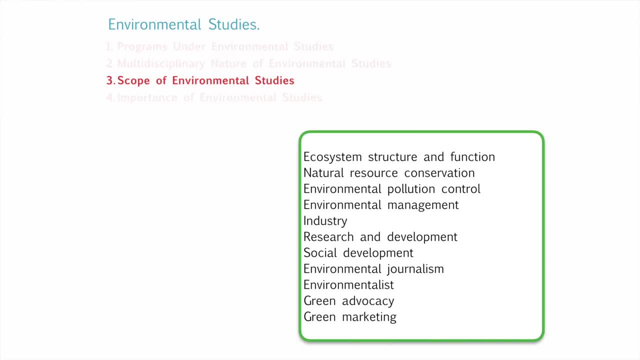 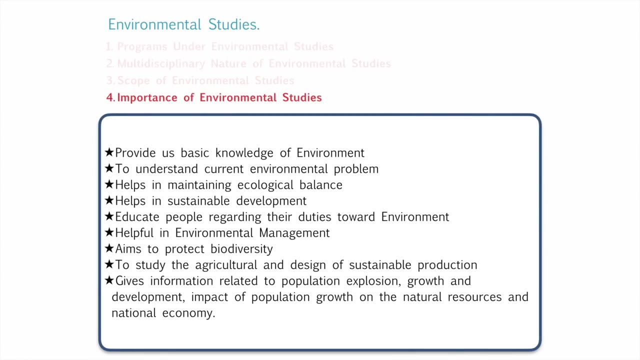 there are a lot of scopes in industry: research and development, social development, environmental journalism, environmentalist green advocacy, green marketing, pollution control, environmental management and many more things are there. now what are the importance of environmental study? the main basic important is to get the basic knowledge of our environment and to understand the current 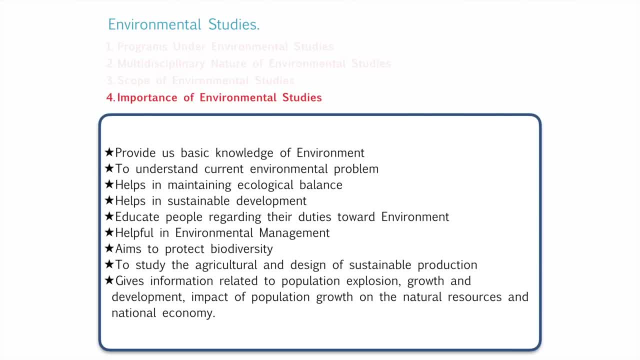 environmental problems, which help us to understand the current environmental problems, to maintain the ecological balance and get sustainable development. we will be educating people regarding their duties towards environment to help the environmental management and to protect our biodiversities. there are so many more importance of environmental studies. 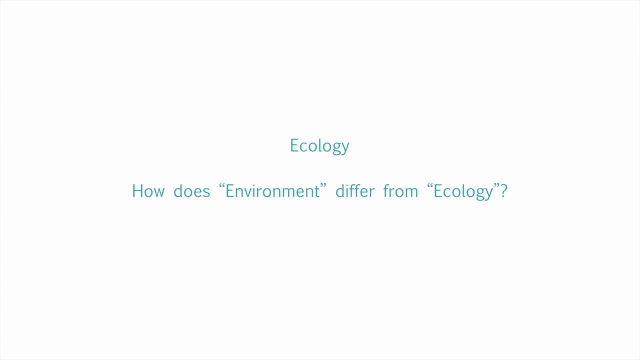 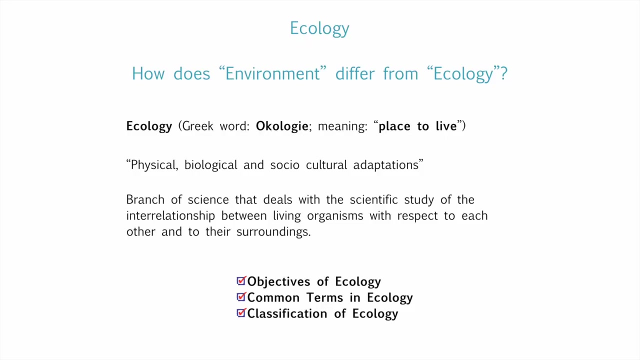 now ecology. what is ecology and how it differs from environment? the term ecology is derived from the greek word apology, which is the meaning of apology is place to live. that means ecology is concerned only about the place where a living organism is living, so it can be physical, biological or social, socio-cultural, cultural adaptations. 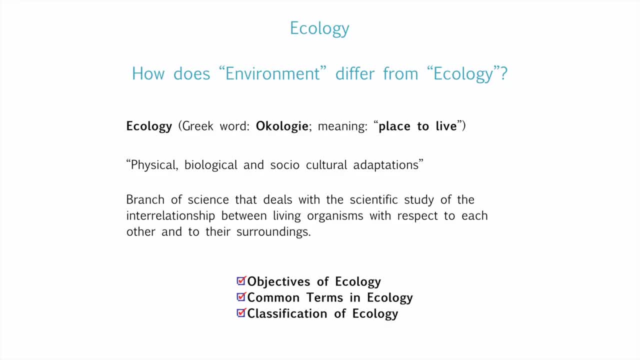 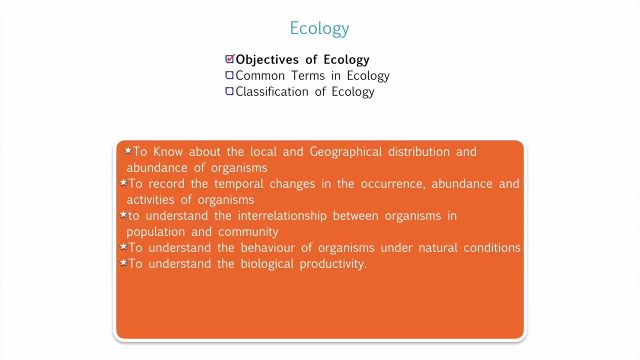 the proper definition for the ecology is the branch of science that deals with the scientific study of the interrelationship between living organisms with respect to each other and to their surroundings. there are three main points to study in ecology. first is the objective of the ecology. so what are the main objectives of the ecology is to understand, to know about the local 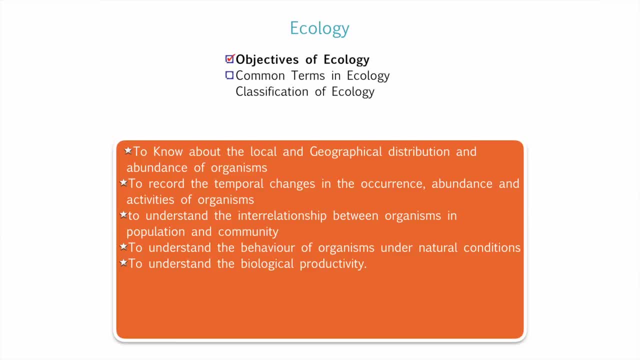 and geographical distribution and abundance of organisms. also to record the temporal changes in the occurrence of organisms- the audience is concerned for the environmental relationship and so on- and activities of organisms. Also to understand the interrelationship between organism in population and in community. Also, this will help us to understand the 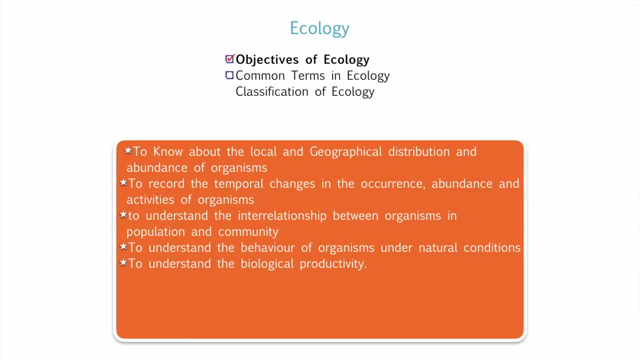 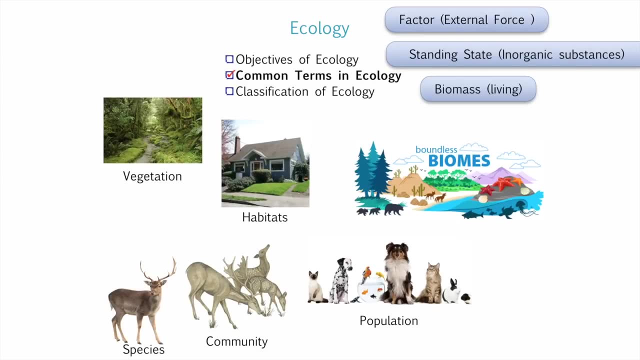 behavior of organisms under natural conditions. We will also understand the biological productivity, Now the common terms used in ecology, which are generally used. So I will just define or try to explain the things. First is the species? Species is a single kind of living organisms, Single kind of living. 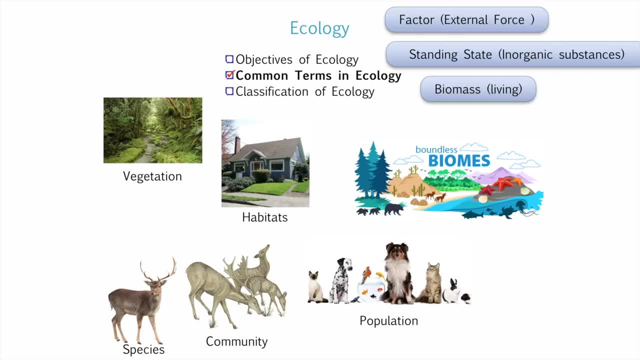 organisms. When the species start living in group, it becomes community. It becomes community, And a group of communities- different communities- becomes populations. Where these populations are living, it's called as habitats, And all this system, including population, habitat and vegetation, forms biomes. Vegetations are the only part of the 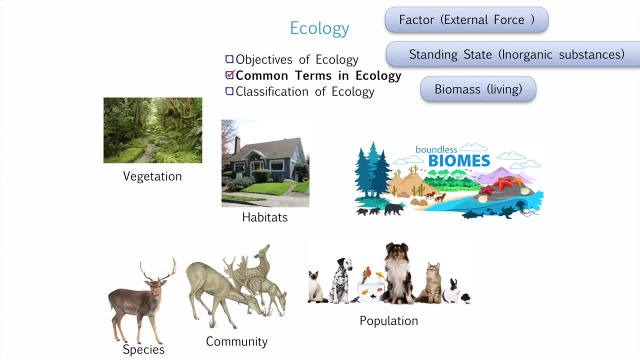 biome, which is involved with only plant materials or plant related studies, And biomes are also divided into two parts, Where all the living material of the biome is the living material of the biome And the living material of the biome is the known as biomass, While the non-living, non-living part of the biomes are. 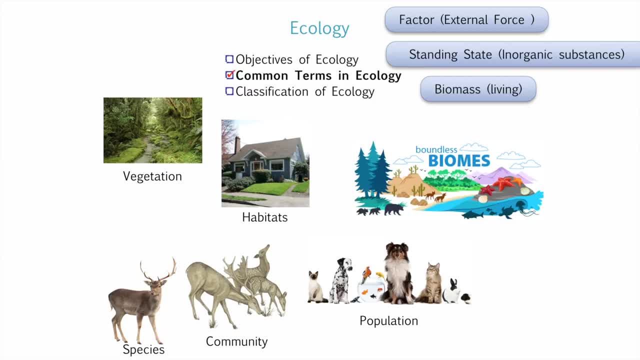 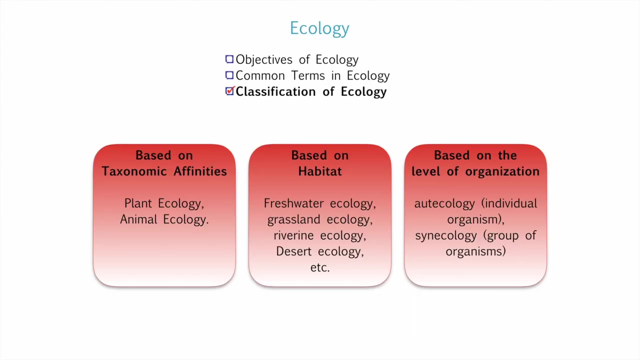 called as standing states, Standing states or inorganic substances. And the factor or the external force or the energy involved in all the processes of the biomes is called as factors. Now the classification of ecology. The classification is based on different types of the different, different methods. 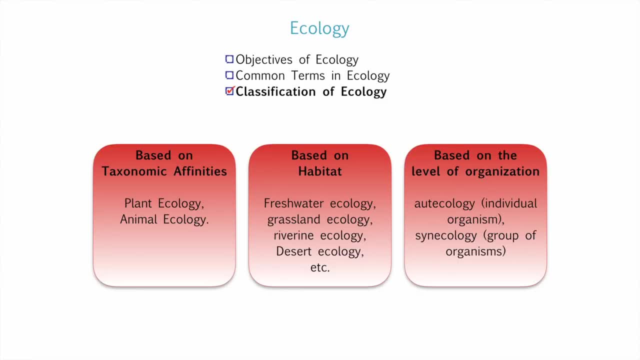 So, based on the taxonomic affinity, they are classified into two parts: Plant ecology and animal ecology. And based on the habitat where they live, It's divided into different parts like fresh water ecology, grassland ecology, desert ecology, river ecology, etc. And based on the level of organization, they are divided into different parts. 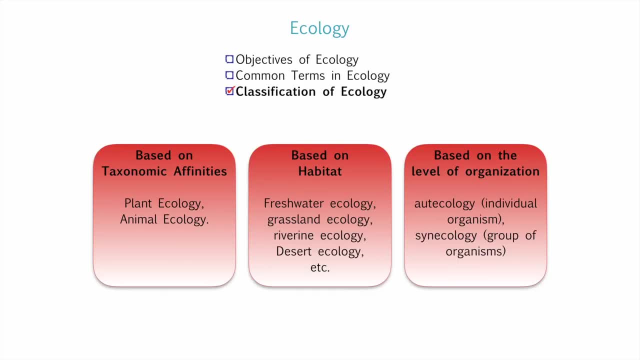 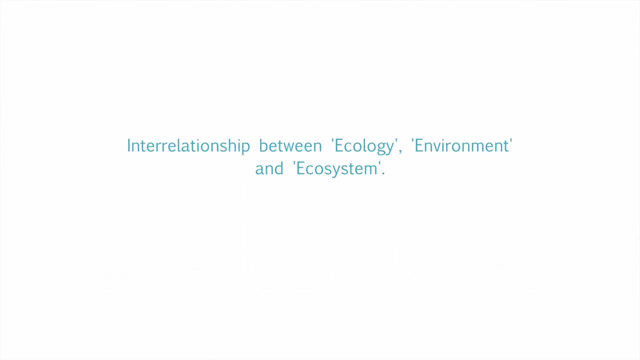 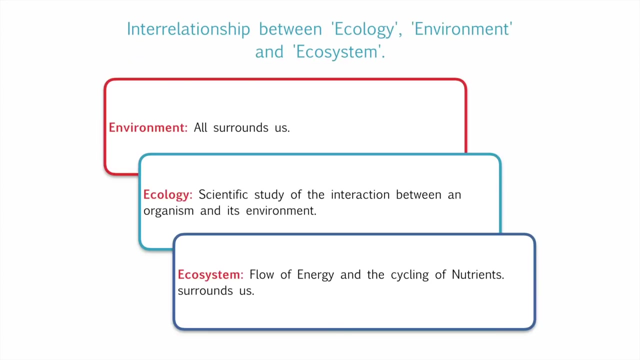 into two parts: Etychology and synecology. Etychology means the living organisms which live independently, individually, and synecology the individuals or the species which live in groups of organisms. Now, the interrelationship between the ecology, environment and ecosystem- Environment, as I already told you, is the all that surrounds us: Ecology. 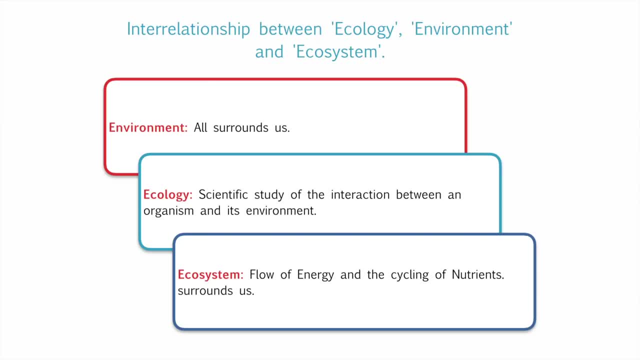 is the specific study of the interaction between the organism and its environment or its living habitat. So ecology is concerned with, only with, the organisms as well as its living habitat, whereas ecosystem is the actual flow of energy and energy and the cycling of nutrients around us, around us, around us. 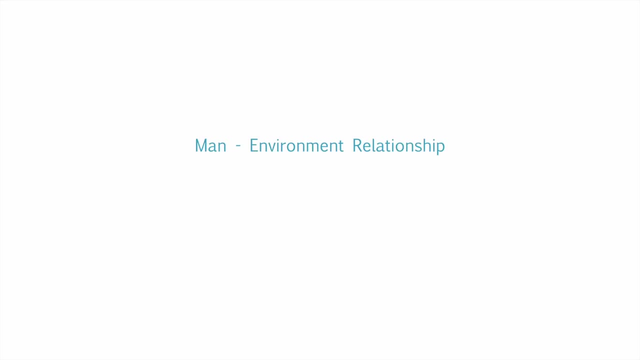 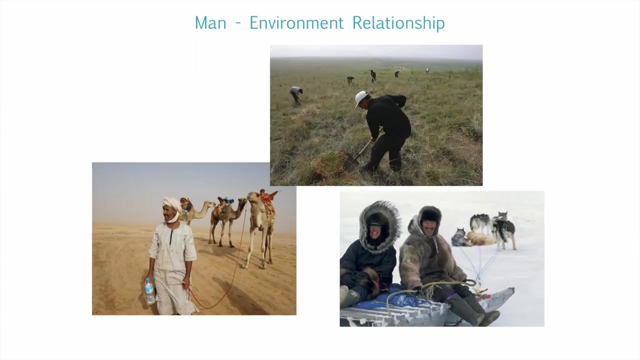 what is the, what is the relationship between man and environment? there is a really great. so the man uses our environment for his different purposes, but also man modifies his environment as required and also man can adopt to different environments. so there is a exchangeable or there is interrelationship between man and environment. for example, the man can adopt to live. 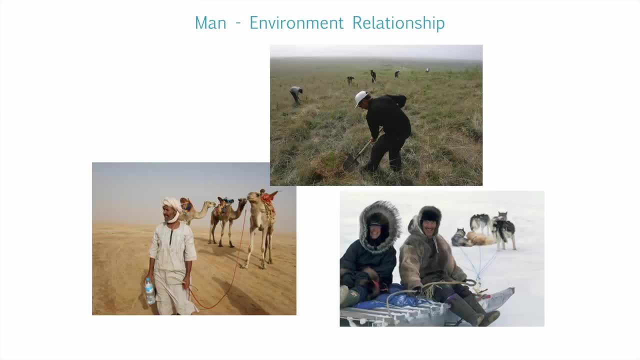 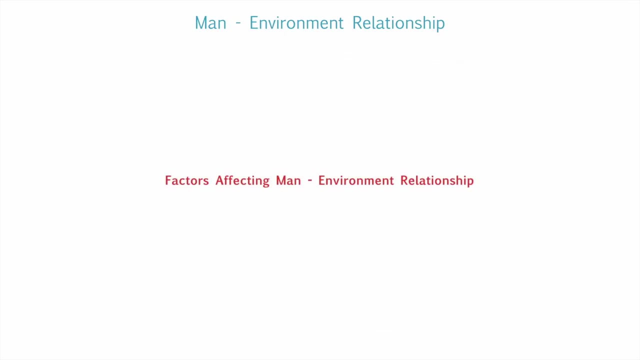 in different conditions, situations like in desert, like in islands, like in grasslands and so many places also. man can modify their environment as per their requirement. they can cut the forest and make the fields as per their requirement, to grow their food or anything else. but what are the main factors affecting the man environment relationship? there are main four. 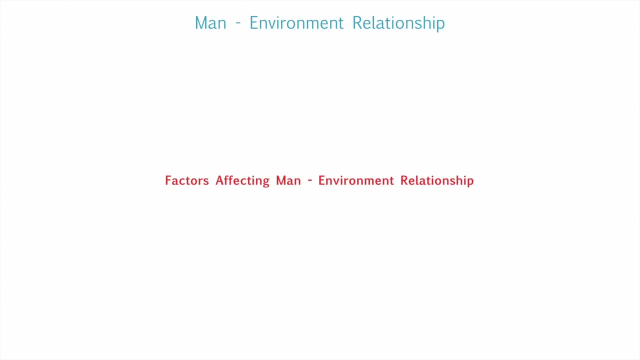 factors which are affecting the man environment relationship. first is growing human population. as the population is growing, we need more and more resources, or natural resources. so we modify our environment as we, as we need more resources. so this is one of the factor which changes the behavior of human beings towards the environment. another is economic development. everybody wants. 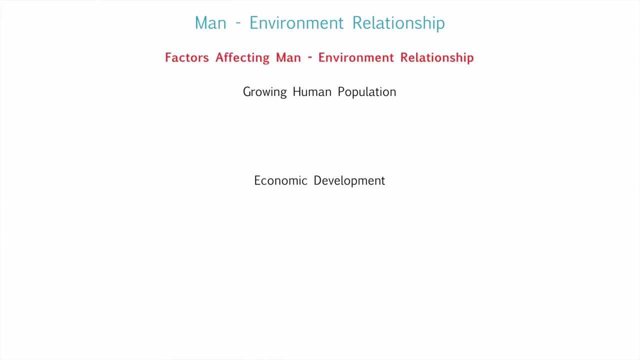 some kind of economic development, and for economic development we modify our environment. we change a lot of things in our environment, so that is also responsible for man environment relationship. next is the consumption of the natural resources. every field, every environment is having fixed amount of natural resources. when they are consumed completely, the behavior of man towards environment changes and he tries to.